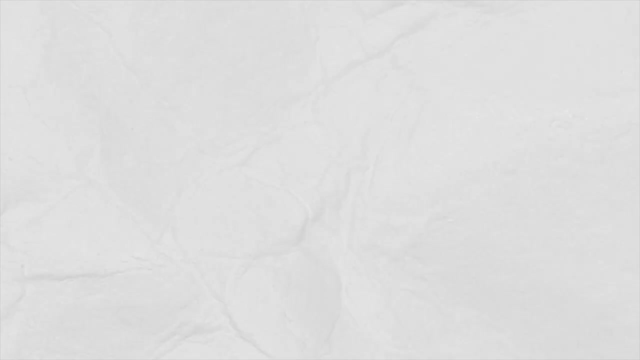 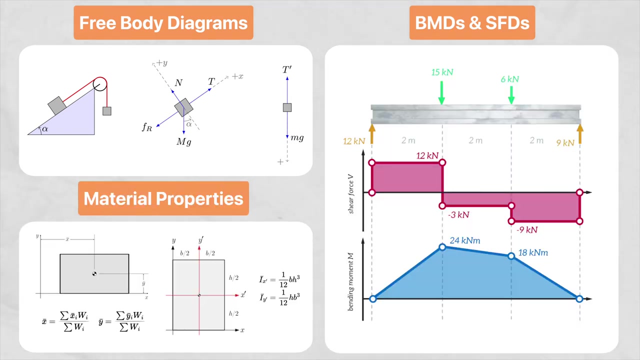 that I would learn is engineering mechanics. Here I would focus on mastering things like solving free body diagrams, drawing bending moment and shear force diagrams, and also how to find and calculate material properties like the center of gravity and the second moment of area. 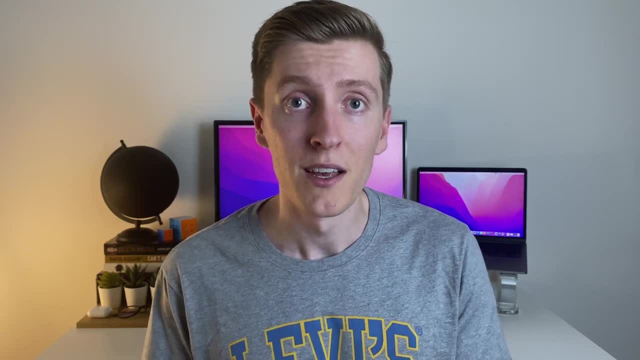 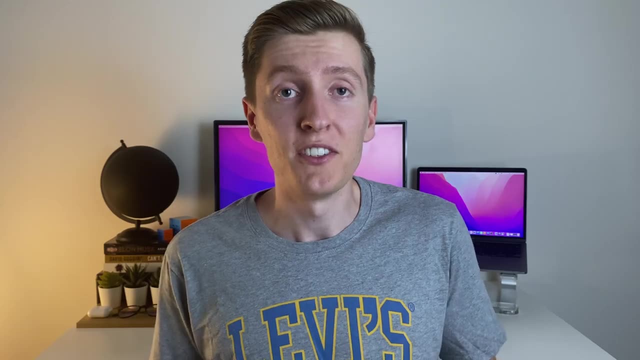 Also, another thing that's important to learn here is the analysis of trusses, of which there are two ways, which are the method of joints and the method of sections. Okay, and next on the list is mechanics and materials And similar to engineering mechanics. 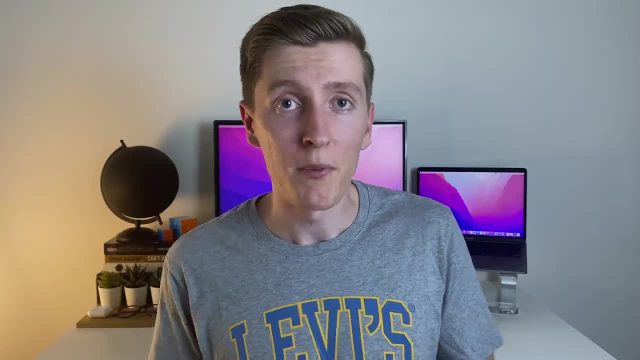 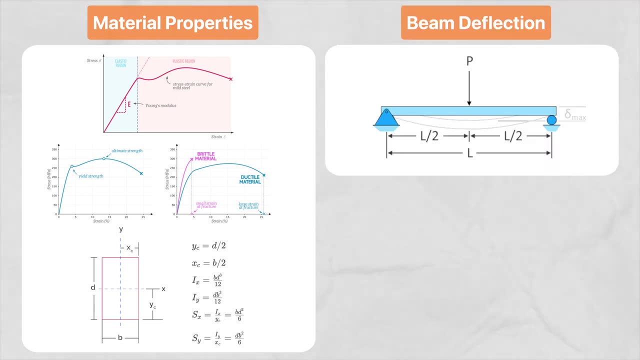 this is all about mastering the fundamentals. Here I would spend my time learning about material properties like the modulus of elasticity and how to calculate the section modulus. I would also spend my time understanding beam deflection and what factors affect how much a beam deflects. And finally, I would learn about how the flexure 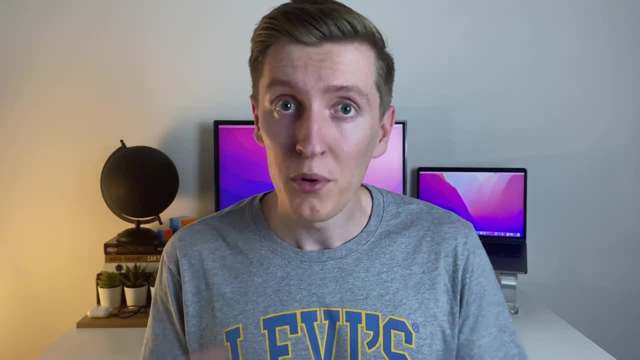 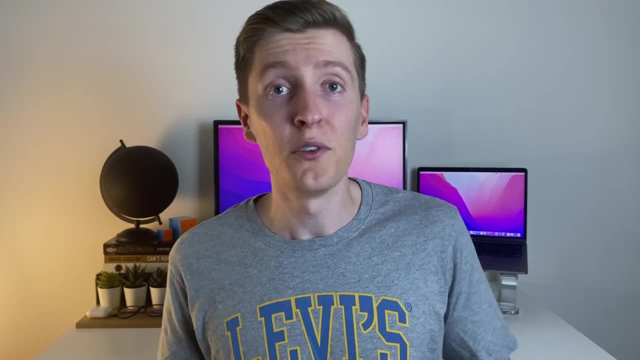 formula works Now, apart from the basics that I've already mentioned, I would not spend any more time than you have to in order to pass your exams, spending time learning how to solve things using first principles. At uni, we spend so much time learning how to solve things using first. 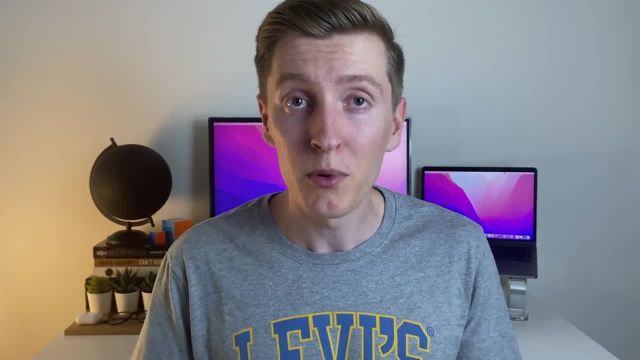 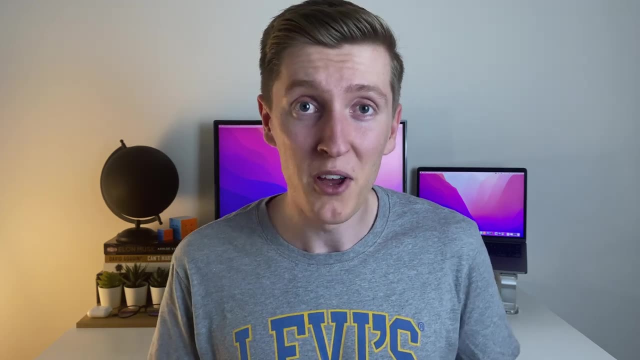 principles, but none of this is actually useful after you graduate, because all of these things have now been programmed into software. For example, once you're a working engineer, you're going to find the deflection of a beam by determining its elastic curve. 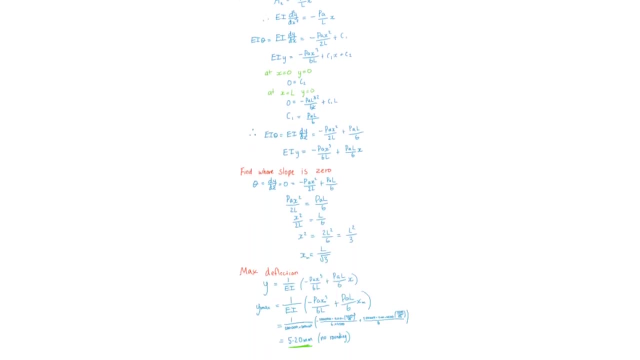 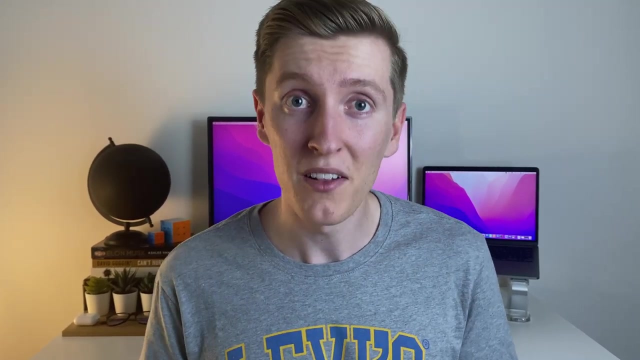 because this involves doing a long-winded calculation that has calculus and algebra in it. Instead, you'll put the beam and its loads into a structural analysis program and then get the result this way, with a lot less effort and a lot less margin for error. 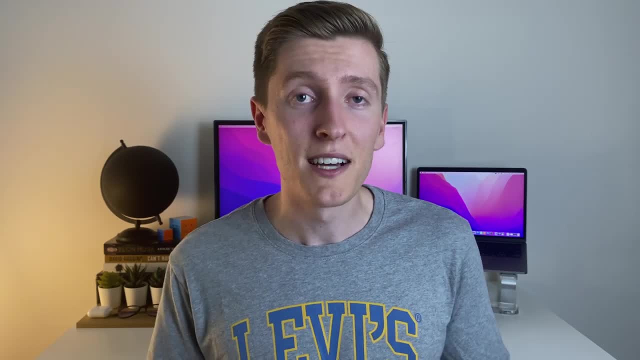 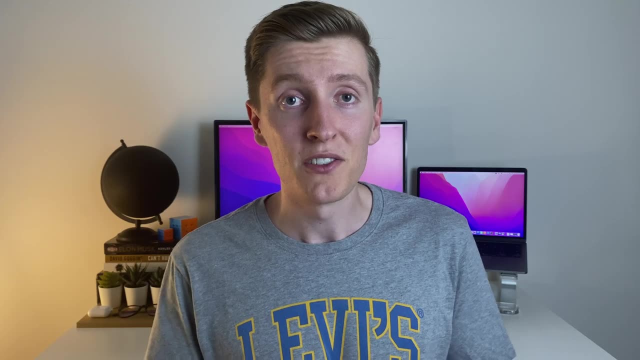 Anyways, after now completing these two fundamental courses, it's finally time to start applying all that you've learned, and the two main ways that you'll do that at uni is by learning steel design and concrete design. Steel design is usually the first design. 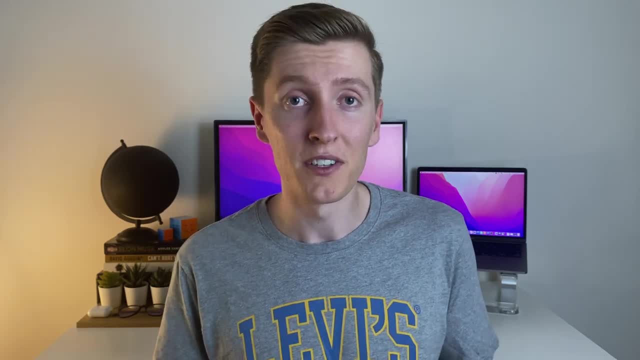 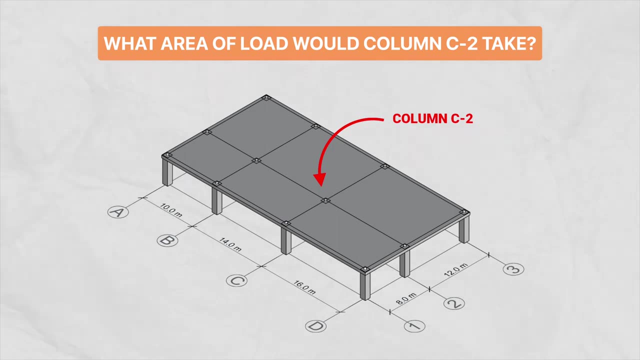 course that you take at uni. so in this course you finally get exposed to the concept of load takedowns, which is a huge part of the job as a structural engineer. A load takedown is basically the process of estimating the magnitude of all the different 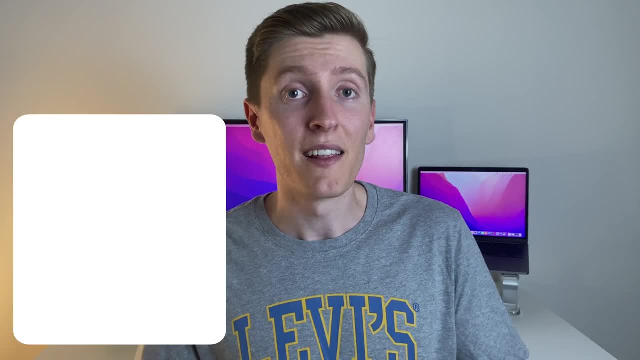 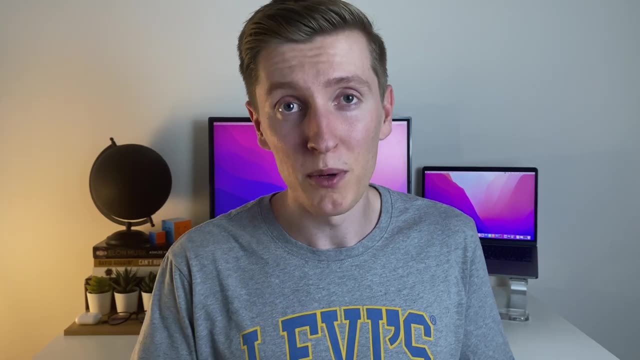 loads that act on an individual member. So this means that you learn how to calculate wind loads, dead loads, live loads, earthquake loads and maybe even snow loads, and then, from here, you learn how to calculate a member's tributary area so that you can apply. 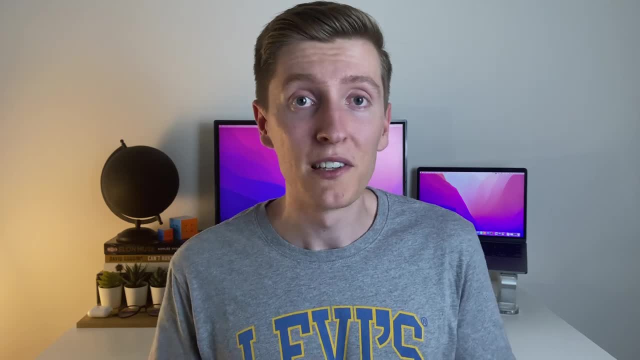 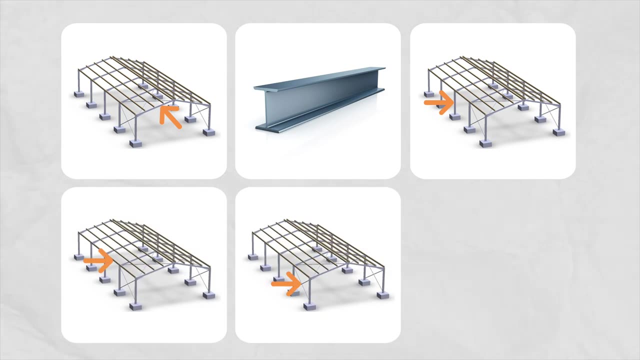 the correct amount of loading. After this you can get into the good stuff, which is learning how to design common steel members like rafters, beams, columns, struts and bracing. Also here you should learn how to design cold-formed steel like purlins and girths. Now designing steel. 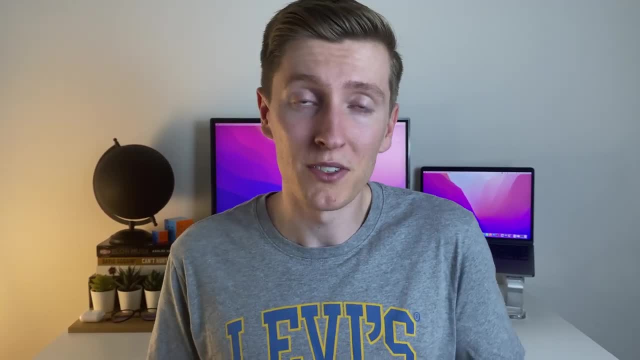 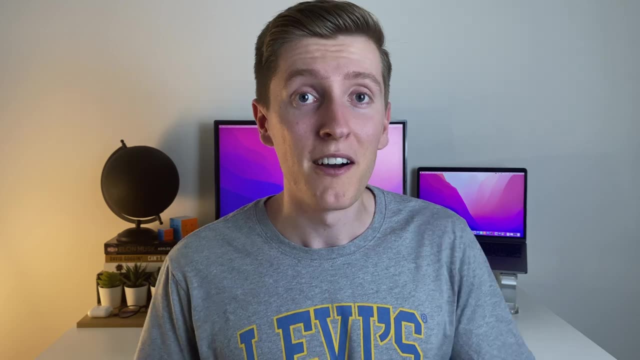 members, is something that you're going to do on a weekly basis when you're a graduate structural engineer, so make sure, once you've got this skill, that you maintain it throughout your studies. Alright, and the second main design course that's really worth your time is concrete design. 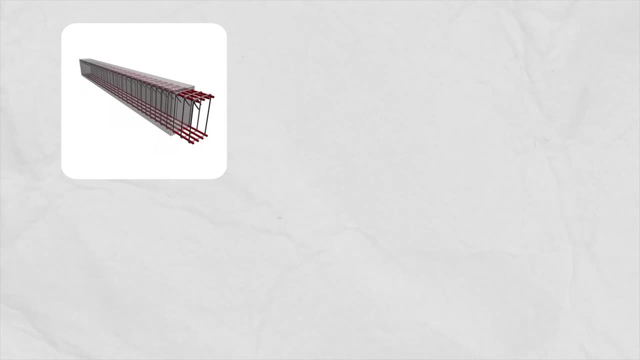 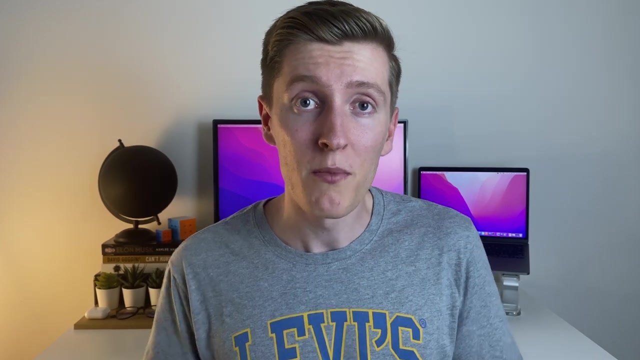 Here you'll learn how to design and analyze reinforced concrete beams, slabs, walls and columns and, depending on your uni, you'll also learn about pre-stressed concrete. In my opinion, concrete design is probably one of the most intricate and technically challenging courses. 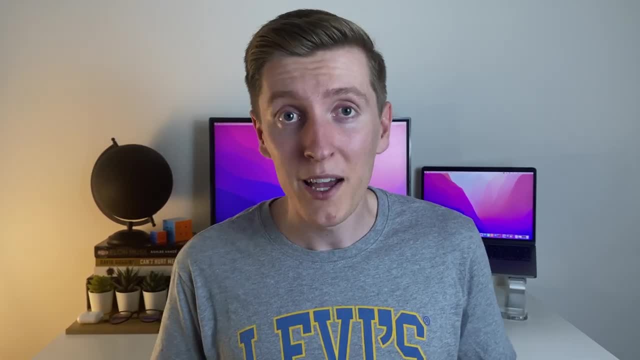 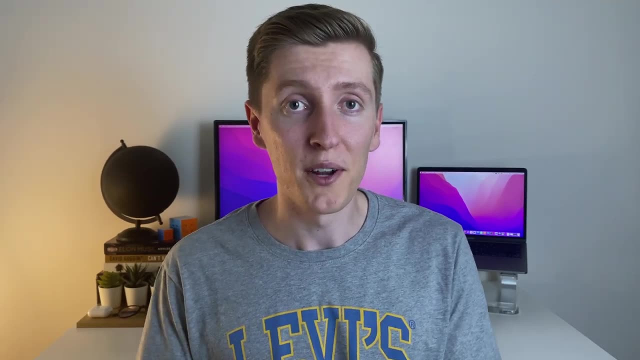 for students, but the concepts are really important to understand, so if you are able to grasp them while you're a student, you will be really well prepared to start working as a design engineer. Alright, so the last thing I've added to the theoretical column is geotechnical. 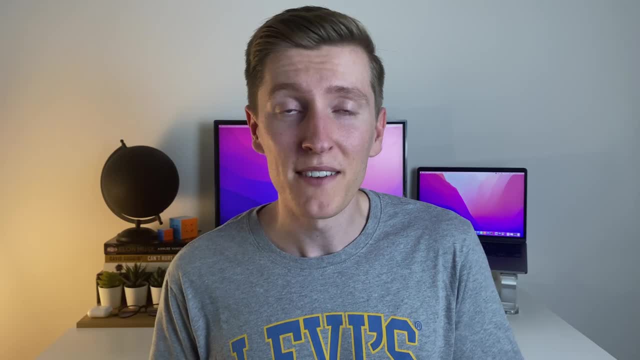 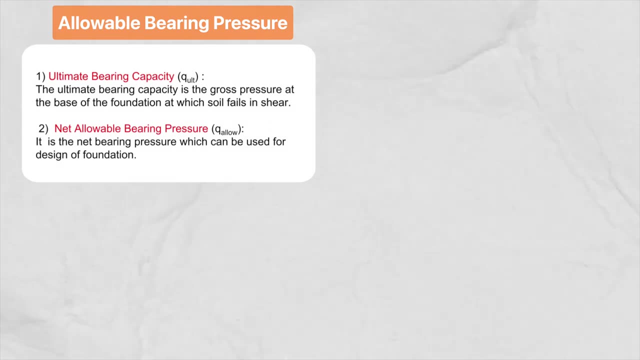 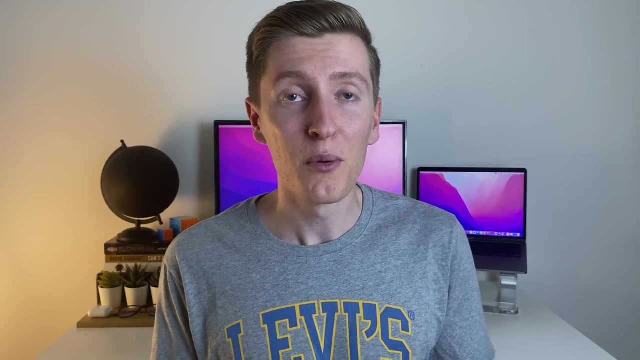 engineering slash soil mechanics. As a structural engineer, you do need to have a reasonable understanding about foundation properties, so the types of things that I would pay attention to here are allowable bearing pressure calculations, soil types and properties, and also lateral earth and hydrostatic pressure calculations for retaining wall design. Okay, so now that we've 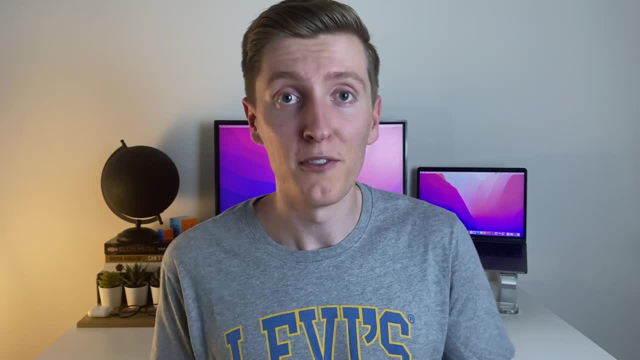 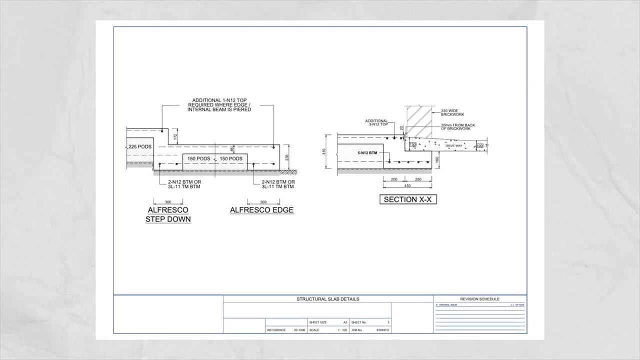 got all the important theoretical concepts, let's move over to the practical column, and first up we have structural drawings. Structural drawings are the final product of all the calculations and analysis we do as engineers, and these drawings are the only thing that builders actually care. 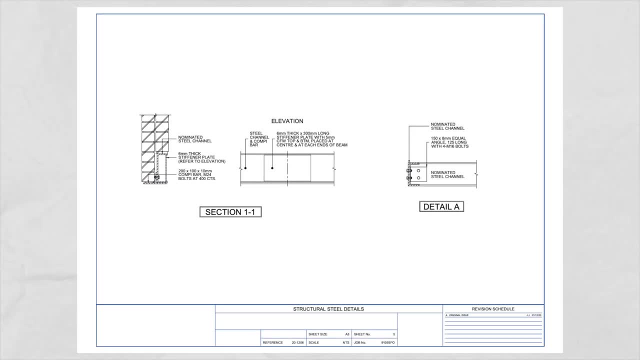 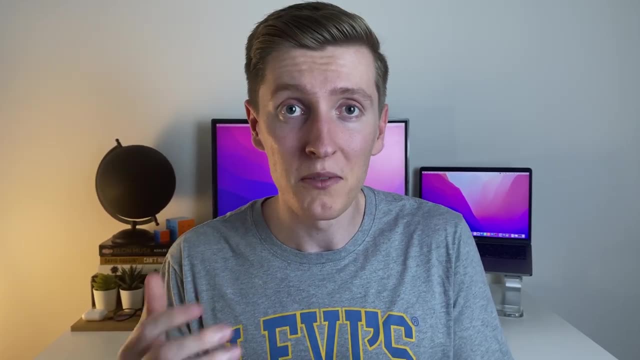 about because they are the detailed picture of exactly what they need to construct. But, funnily enough, at uni no one teaches you how to read or even make these drawings, And although learning how to make these drawings is something that you can master over time when you start working, 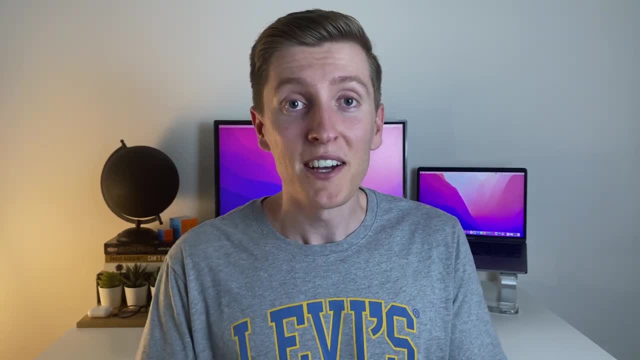 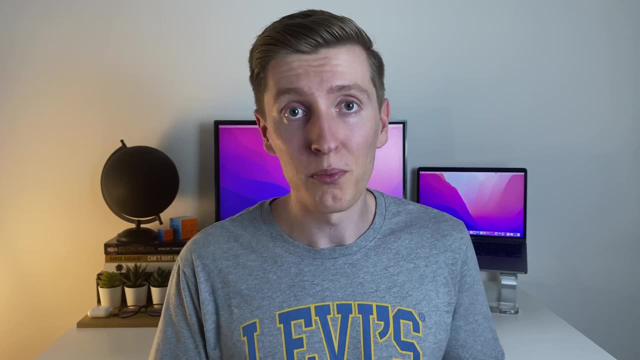 learning how to read these drawings is something that you can master now. I've actually already on my channel about how to read structural drawings and if you're learning from scratch, like I was watching, that video is a good place to start, but eventually you're going to need to. 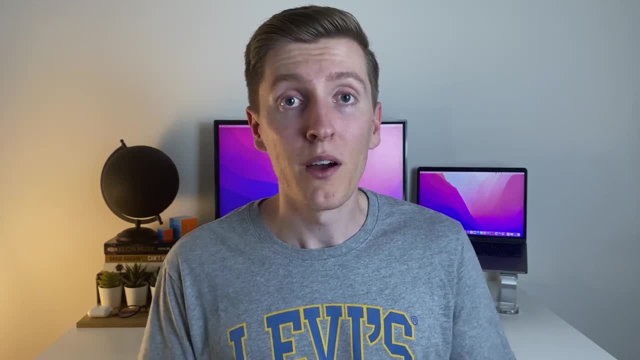 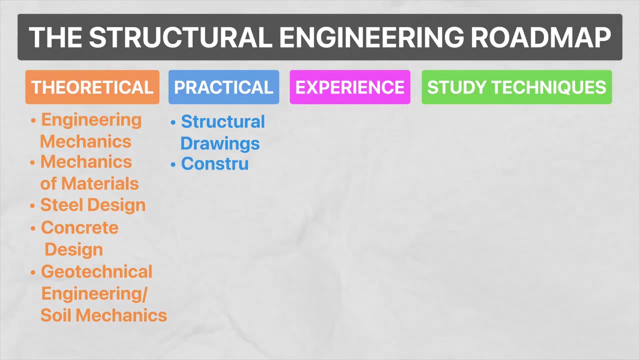 get your hands on a set of drawings and then just do some practice. So I would suggest getting on google and doing a search for a set of structural drawings and then just getting familiar with how things get displayed and referenced. Okay, next on the list is construction terminology and what I 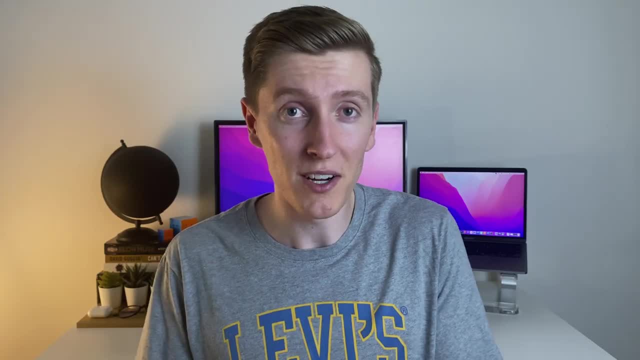 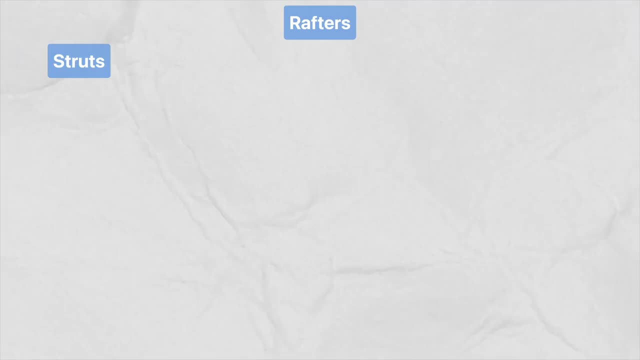 mean here is learning the names of as many different things that are used in construction as possible. For example, a few of the building components that you'll need to be familiar with are rafters, struts, racing outriggers, purlins, flats plates, fin plates, cap plates, t-clates. 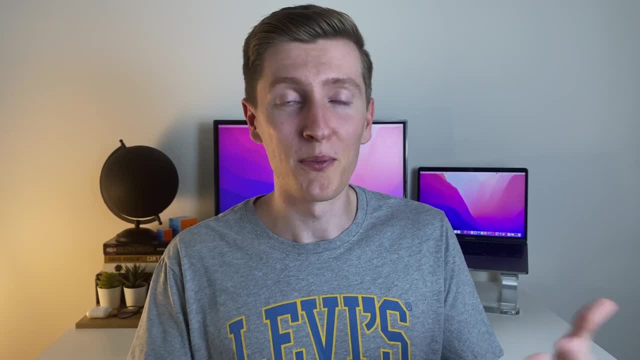 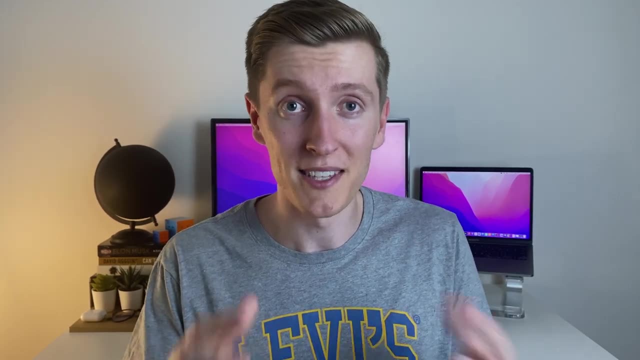 stiffeners, fillet welds, butt welds and bolt sizes. Okay, that was a bit of a joke, but I think you get my point. There's a lot of different things that you need to learn the name of in construction, and by simply turning up to class you're not going to learn those things, So what? 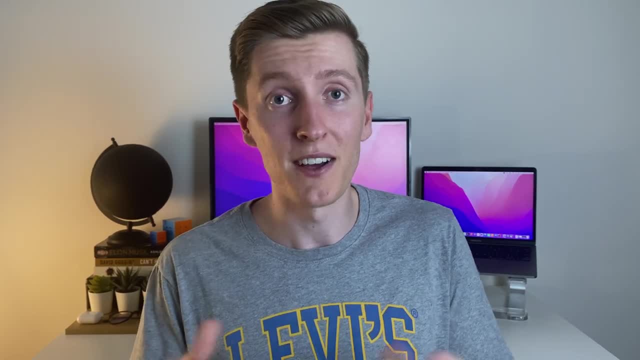 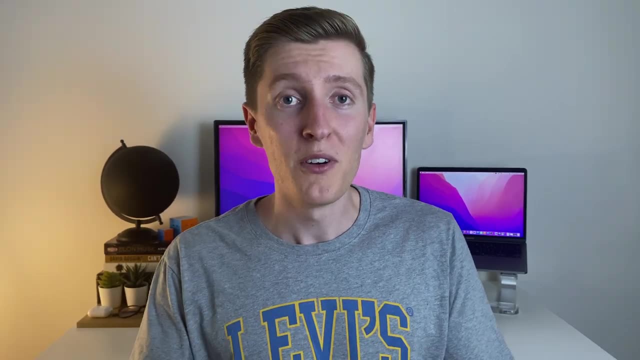 I would suggest doing is getting on google and searching up annotated diagrams of timber, concrete and steel construction and trying to commit as many of those names to your memory as possible. One of the most overwhelming things as a graduate engineer is when people are constantly. 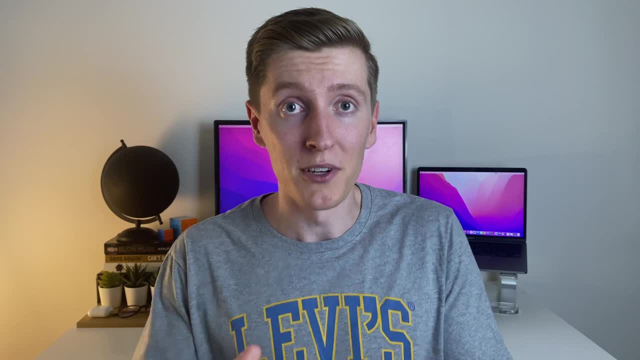 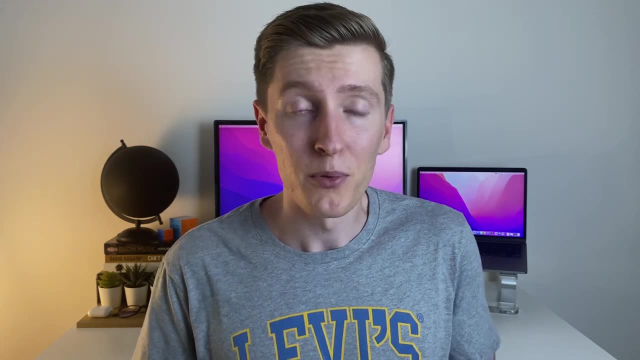 talking about things that you have no idea about. so this is one of those processes that will definitely pay off big time. Alright, and next on the list is software programs. Obviously, these days, analysis and design programs are a huge part of every engineer's workflow. 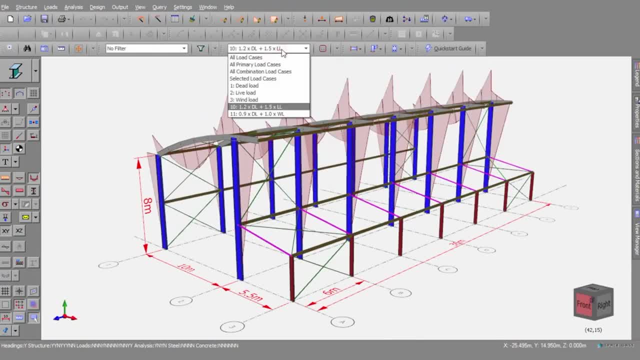 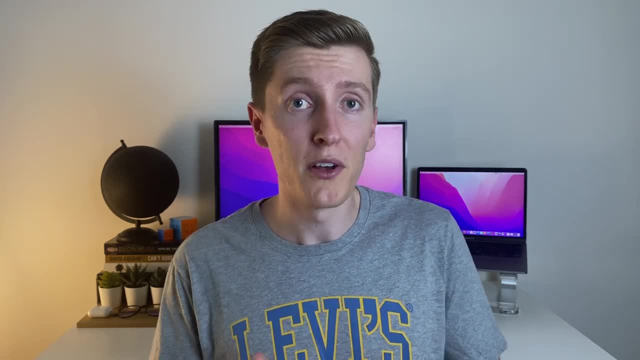 so learning how to use these programs is not only going to make you a lot more employable, but it's going to make you a better engineer. Now, if I was going to be learning how to use these programs from scratch, the four programs that I would learn how to use, because they're 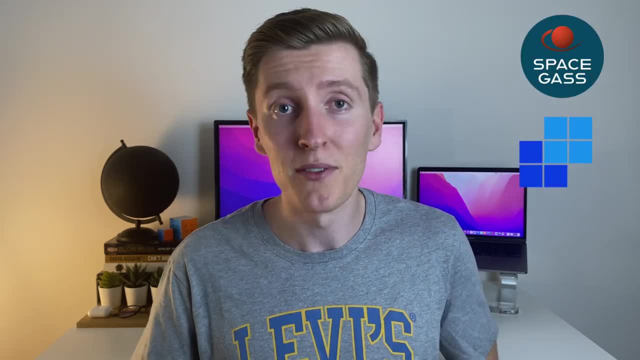 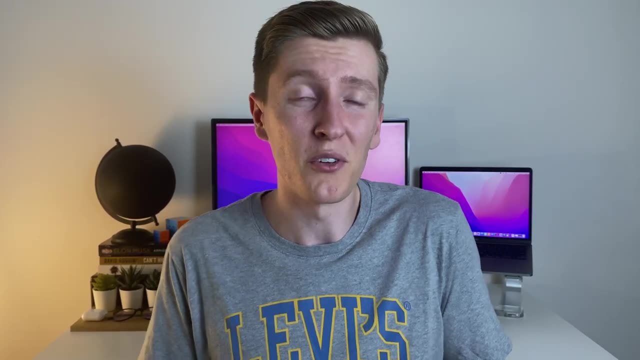 the most relevant to me today are Space Gas, Strand 7, Ram Concept and Wrapped. These particular programs may not be popular depending on where you live, because it tends to change depending on your region, but as long as you're getting familiar with some sort of steel, 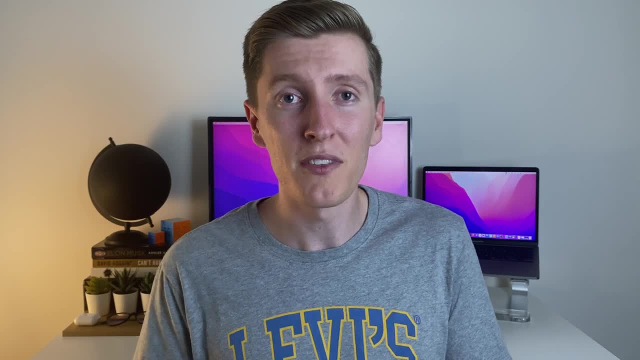 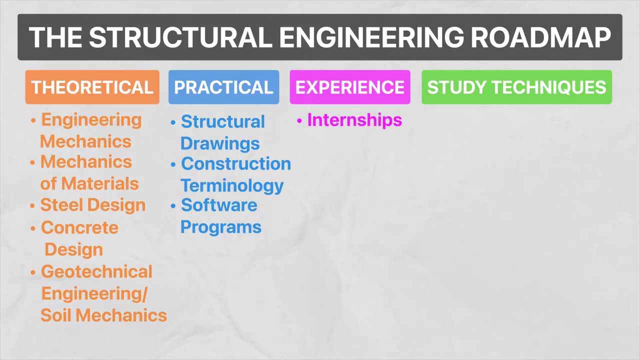 design and concrete design program, you should be fine, because a lot of the skills are transferable to other programs. Okay, and now it's time to move on to the next heading, which is experience, and first up is internships. Knowing what I'd do now, the advice I'd give to my younger self, 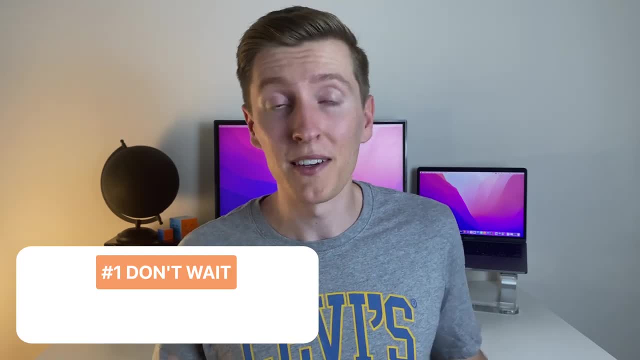 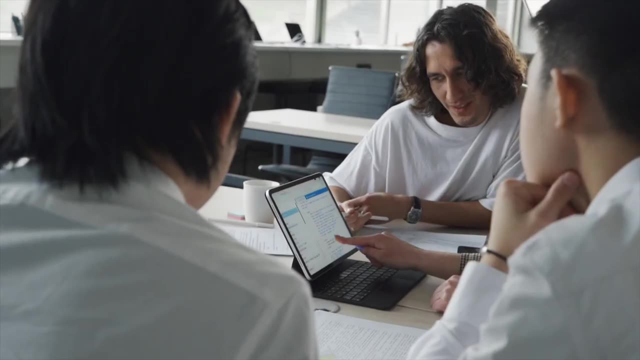 regarding internships is: one: don't wait, start applying for internships in your first year of uni. and two: only target small companies. The reason I'd give myself this advice is because I think that being able to consolidate the things that you're learning by working on real projects, 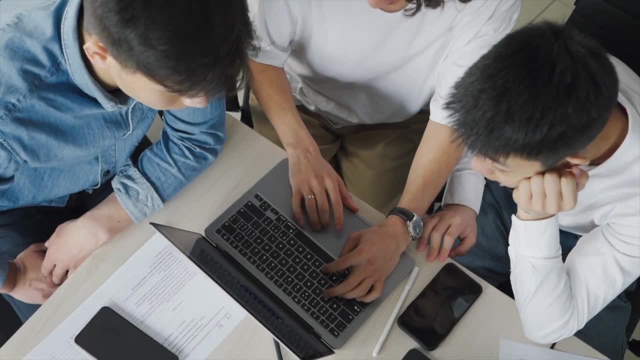 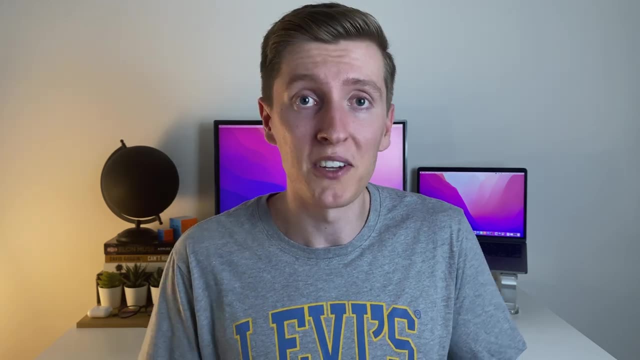 while you're at uni is going to be able to allow you to see the bigger picture and is also going to make you so much more proficient at your job when you start working as a graduate engineer, because you already have a few years experience under your belt, And also the reason I'd tell. 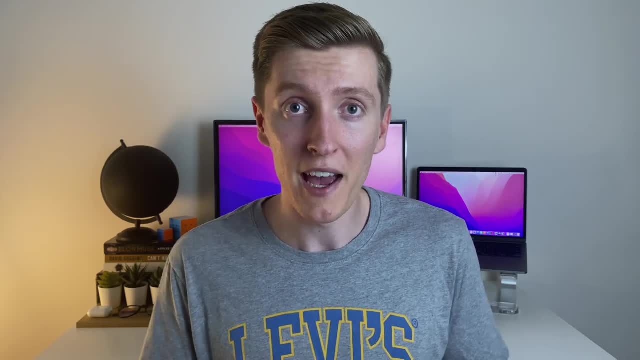 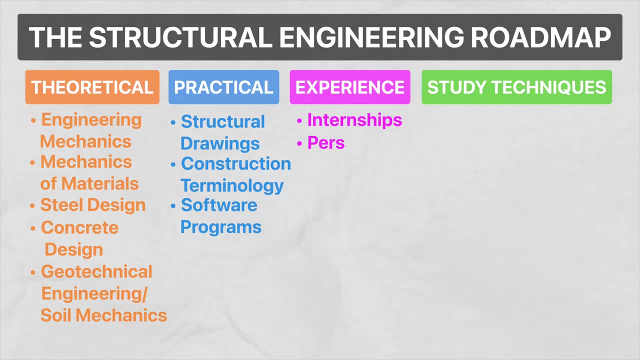 myself to target smaller companies is because in these atmospheres you're able to get a lot more hands-on and the mentorship and the teaching you get here will far outweigh anything you can get at the larger companies. Alright, and the other thing I have in this section is personal. 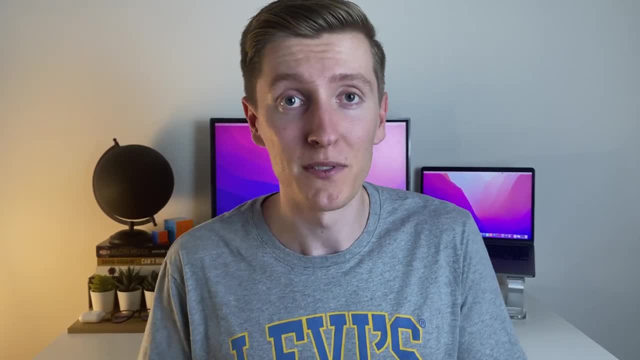 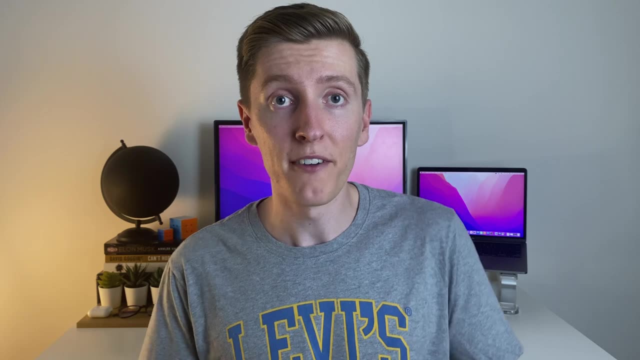 projects, and what I mean here is simply trying to design different types of structures by going through the whole calculation process and then trying to produce a structural drawing. In some of your university classes, you'll have projects where you need to design simple things like a. 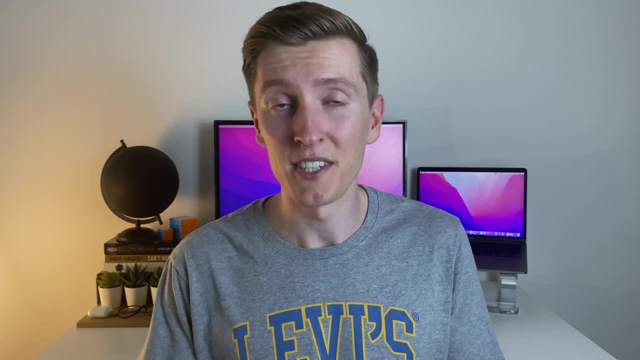 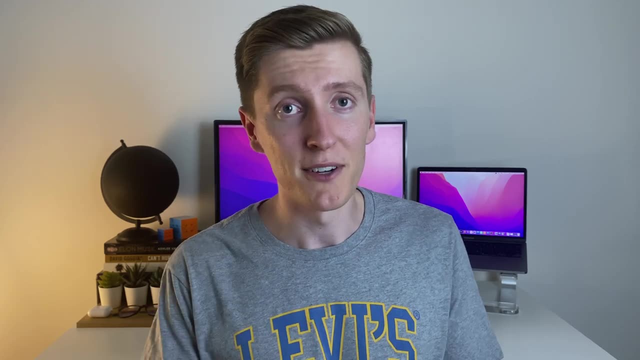 signpost or a portal frame, but you'll rarely have to go the extra step and produce a structural drawing. But if you really want to improve as an engineer, these are the sorts of projects and tasks that are really going to make the difference. For example, if you've already taken the steel.